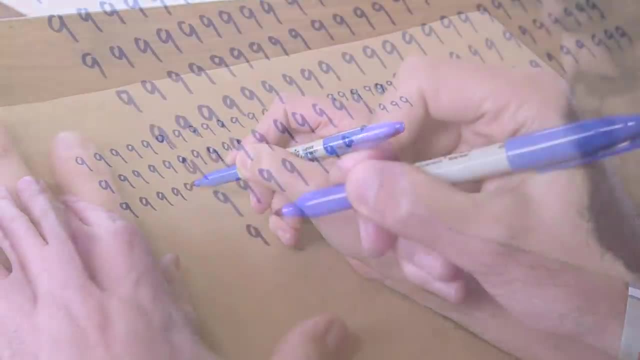 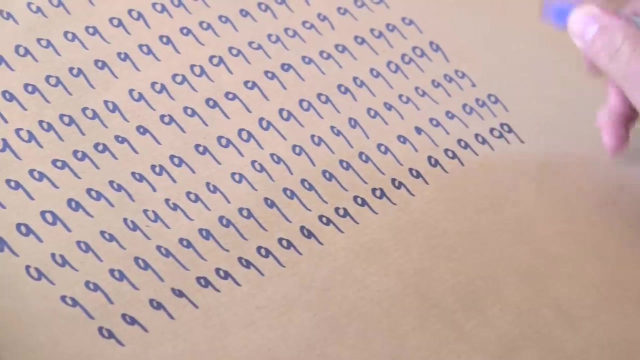 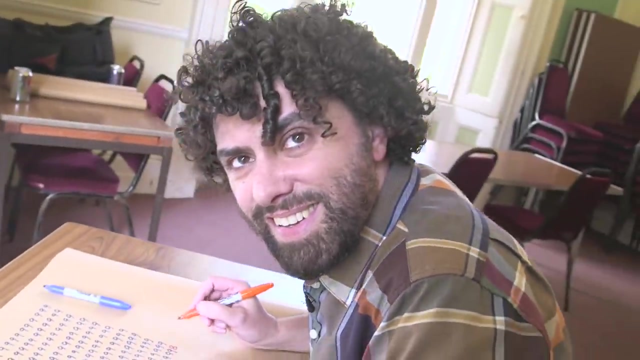 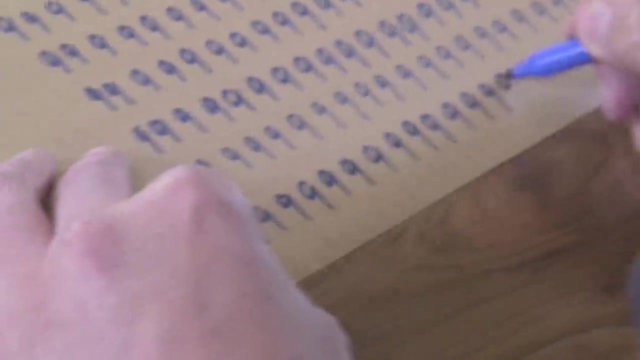 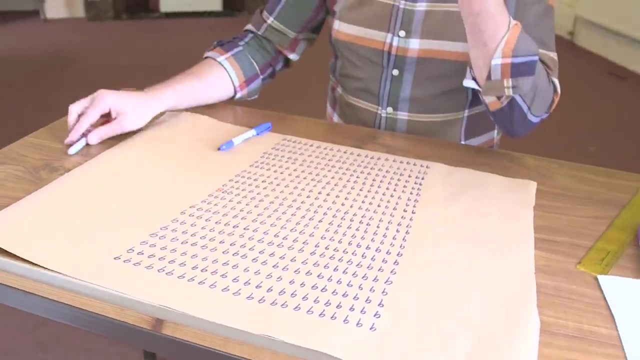 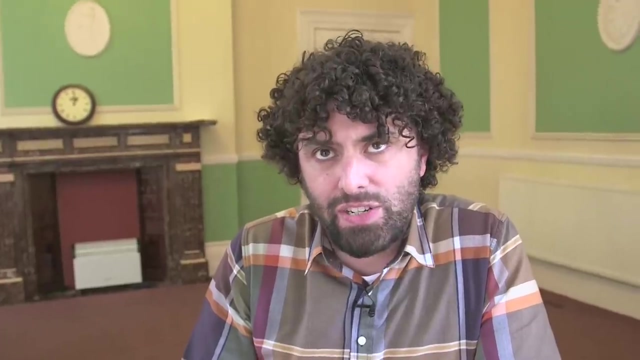 you, Here we go, Here we go, Here we go. Whoa, And in the words of Andrew Wiles, I think I'll stop there. This number here, all nines. you can see it. In actual fact, the way that you'd describe this is as a rep digit. So 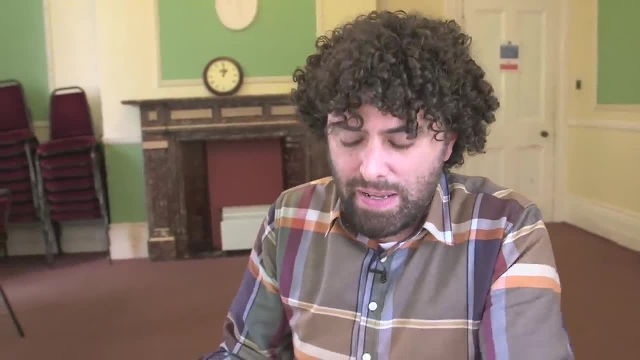 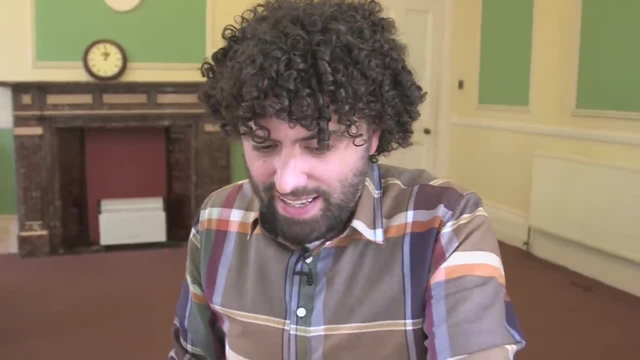 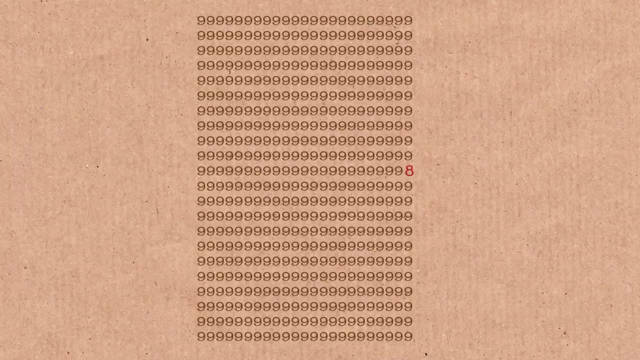 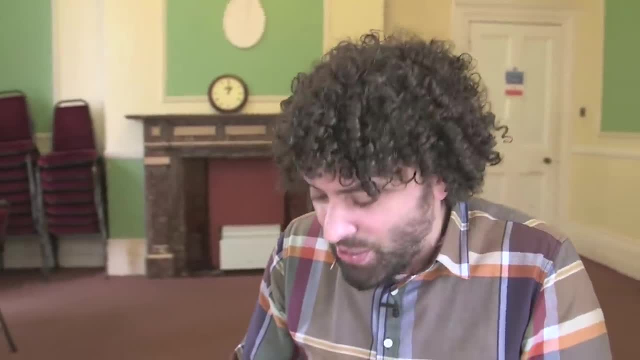 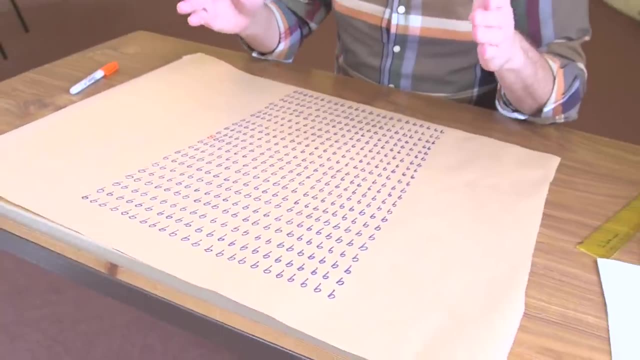 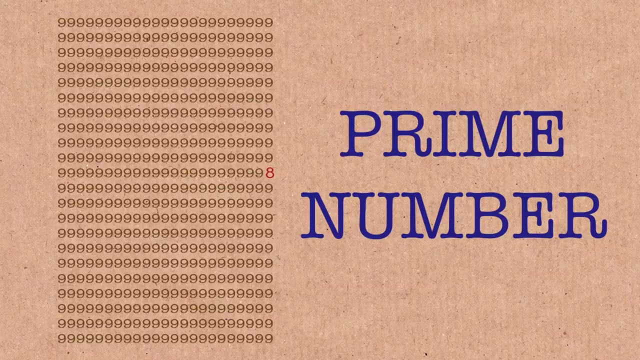 really close. But you know what I like to call it, Brady, I like to call it a glitch. I feel like it's a glitch because it's not only a glitch number. Believe it or not, this is a prime number. This here. I posted this on Twitter. It really got people going, But you know what I thought. 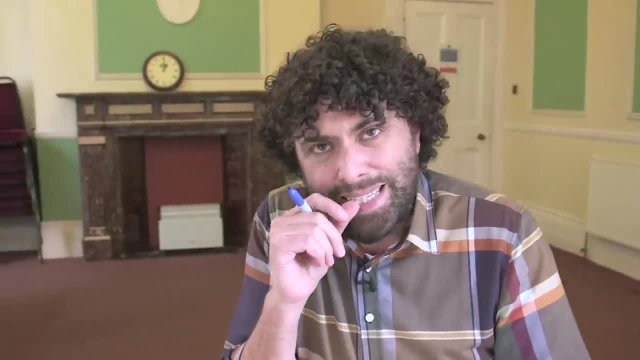 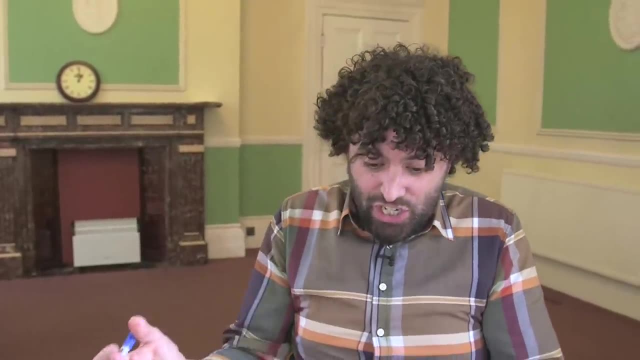 Brady, I thought you sure they haven't made a mistake. I'd really like to check this number. you know, as a mathematician, that's what you want to do. you want to check it. the only problem is: how do you check a number like this? I really don't. 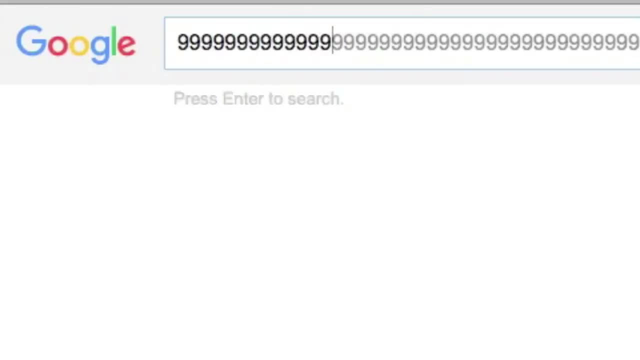 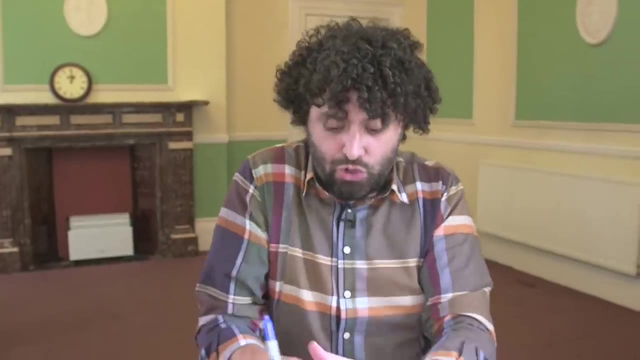 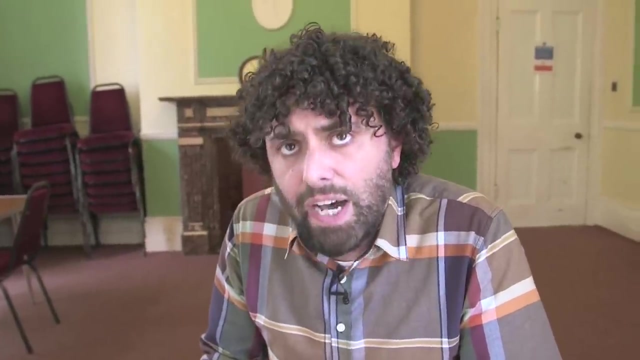 suggest you stick this into the, the Google entry line, to actually work out if it was a prime or not. I actually needed to compactify it. I mean, I needed to actually go. I needed to actually transform it into something that I could carry around. so this number has 506 digits, and so the eight here is actually 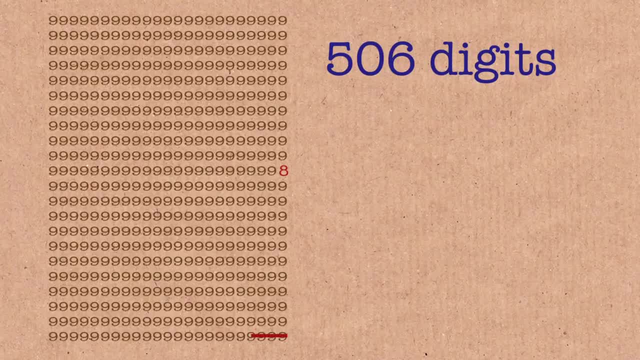 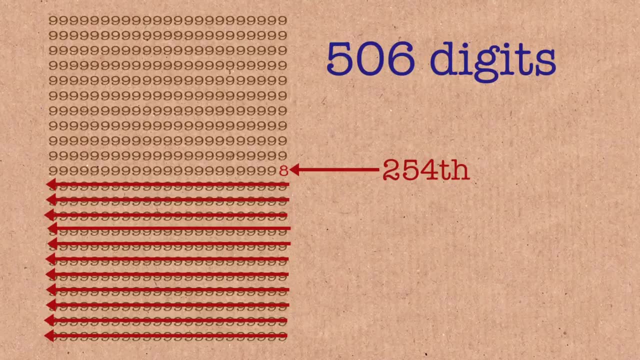 if you count from the bottom, from the ones column and the tens column and the hundreds column, if you get up you'll actually get to the 254th column. so it's actually 254 along. so it's just over the halfway. how can we actually transport? 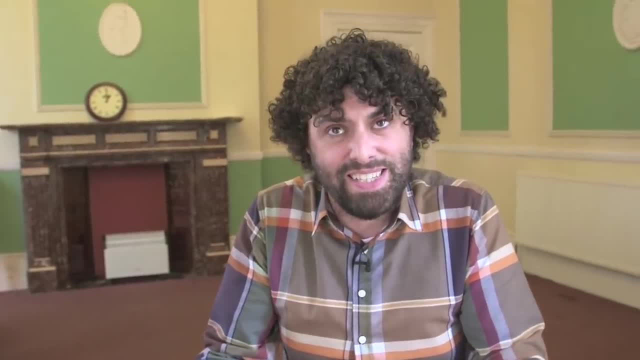 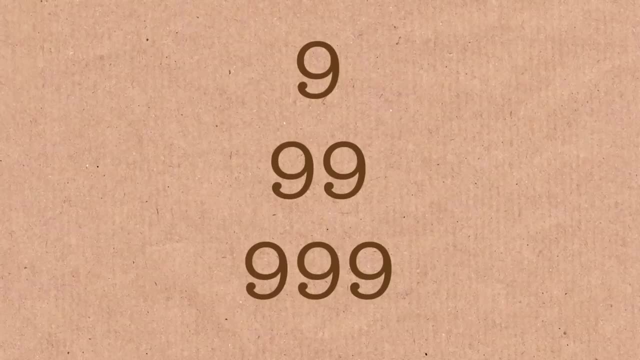 this in a way that doesn't involve me writing out all these nines in any ideas. what's really cool about it is the fact that they are nines. so if you add 1 to 9, you get a 10, and if you add 1 to 99, you get a hundred. and if you add 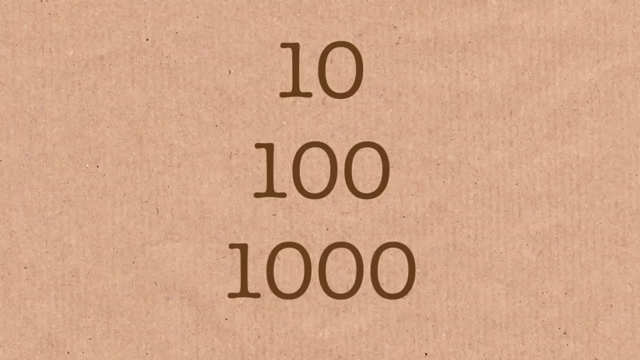 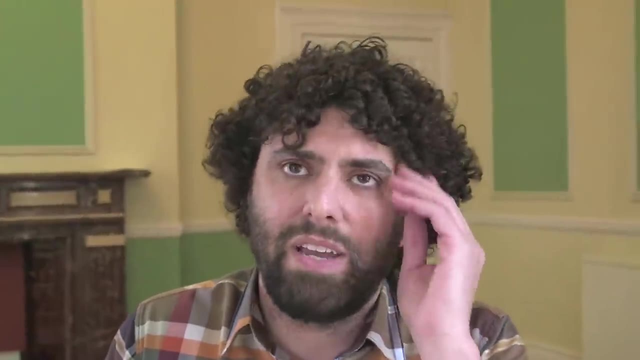 1 to 999, you get a thousand. so we can actually use that fact, because if we can actually get this as something to the power of 10, well that can really make things a lot easier for us to handle. so, if we think about it right, this has 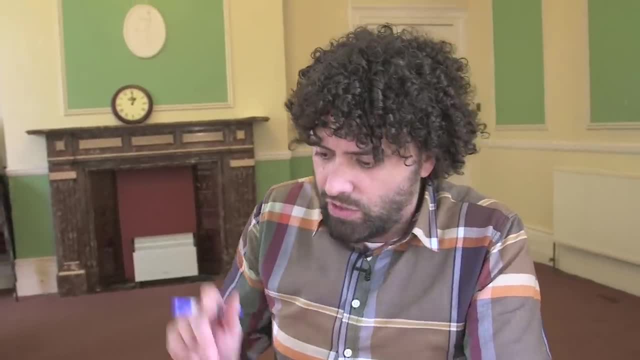 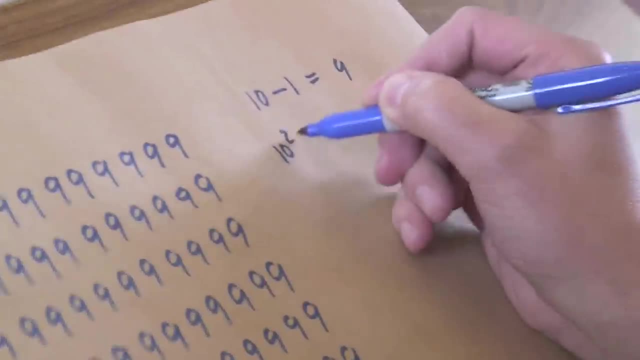 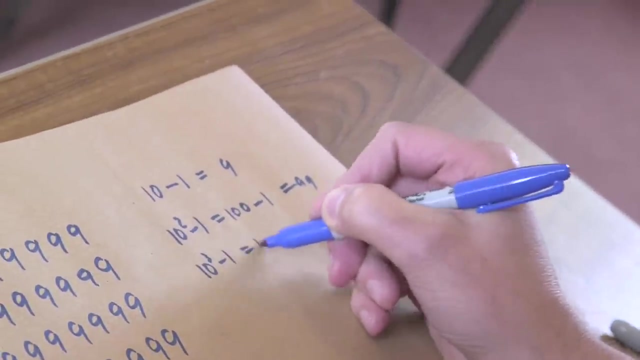 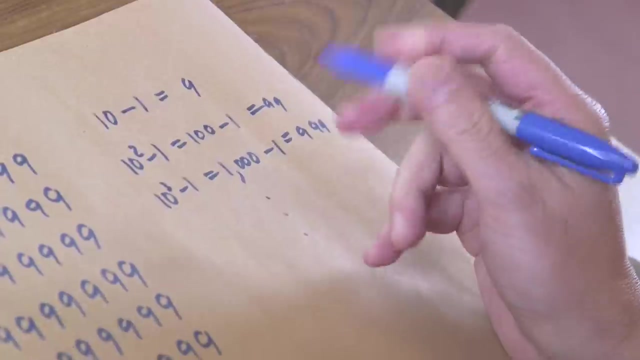 four, five hundred and six nines. so if we say 10, take one is nine, 10 squared, take one which is a hundred, take one is 99 and 10 cubed, which is three zeros there, take one is nine, nine, nine. then if we go dot, dot, dot and you've got to love the dot. 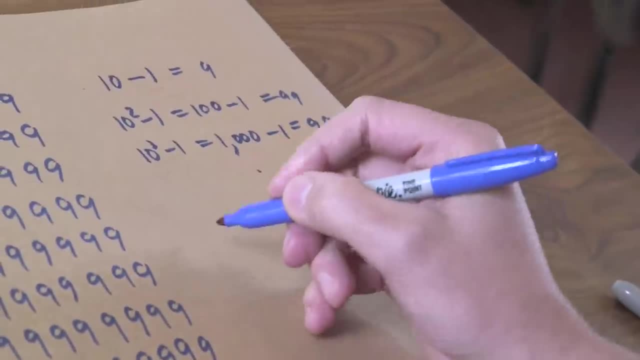 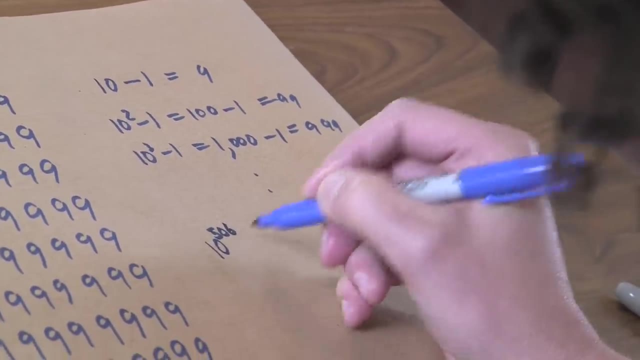 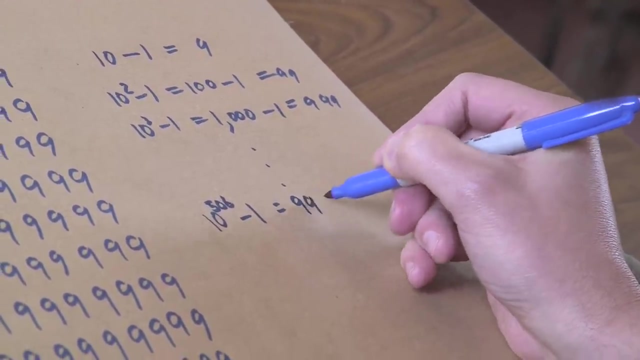 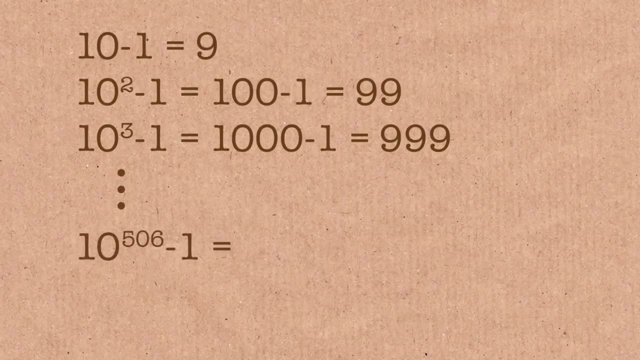 dot dots, because you can put anything in dot dot dots. we can then say ten, two, the five, zero, six. take one is equal to: let's just jump to the chase, hey Brody. is equal to nine, nine, nine, dot dot dot, nine, nine, nine, where this happens to. 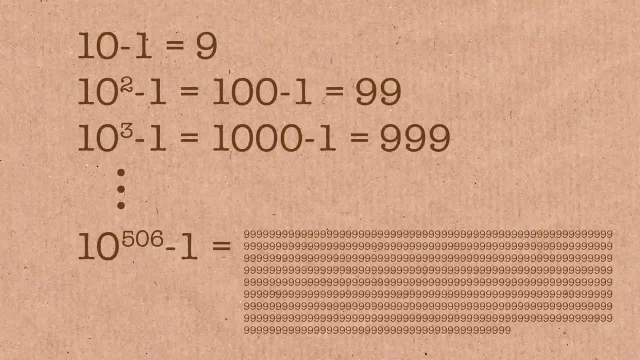 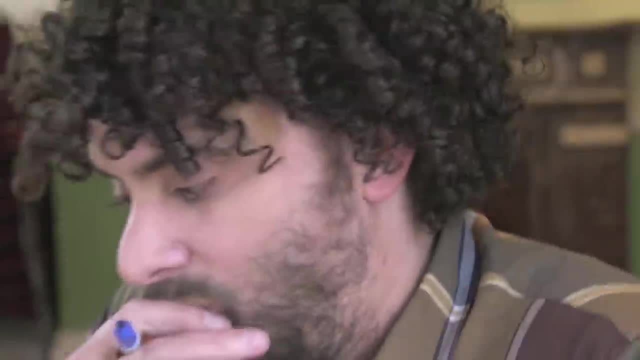 be 506 digits. so that's kind of that. except for that, i know it's a small change, but that actually changes with the way it's written. Yes, Changes the value of the number quite a lot, doesn't it? What do you mean? changes the value. 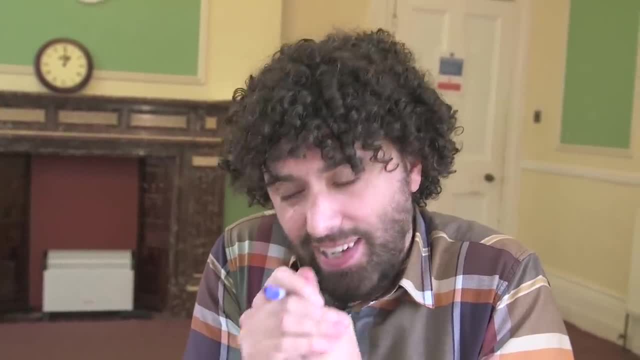 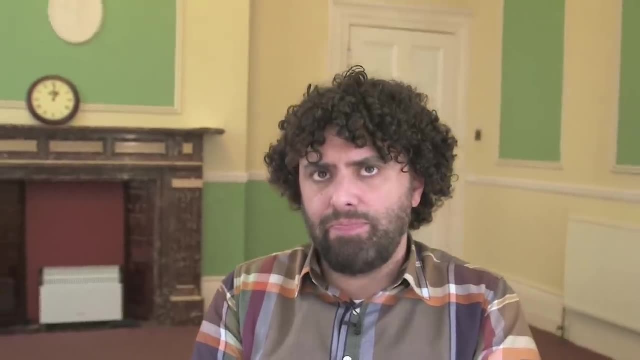 The quantity, Like, if you were going to buy that many eggs, You were going to put this into eggs. Changing that from an eight, Changing that from a nine to an eight, would dramatically change the number of eggs you just bought. Well, you know what? 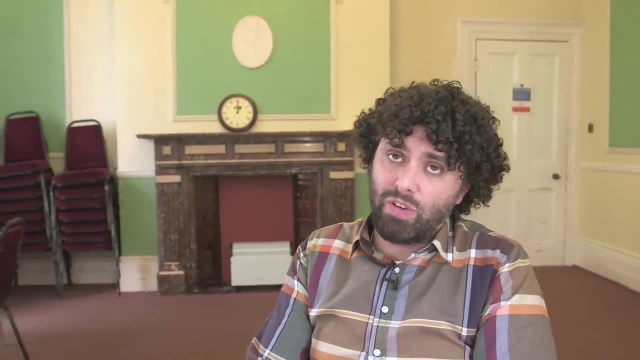 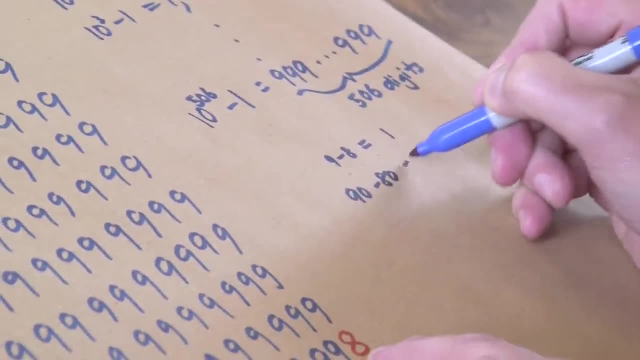 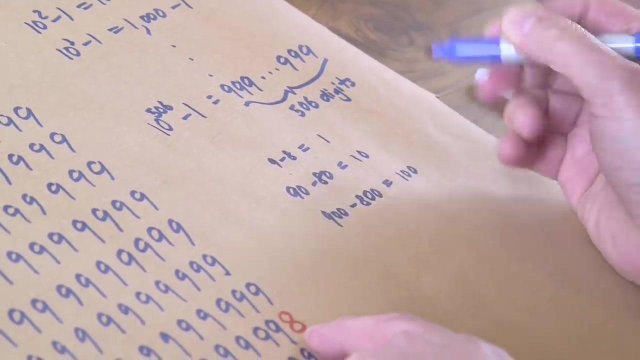 You're exactly right. And to actually work out by how much you're actually solving the problem: Nine take eight is one. Ninety take eighty, that's ten. Nine hundred take eight, hundred is one hundred. Can you see the pattern going on here? 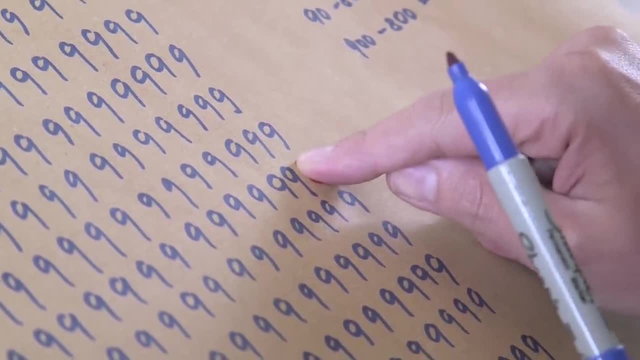 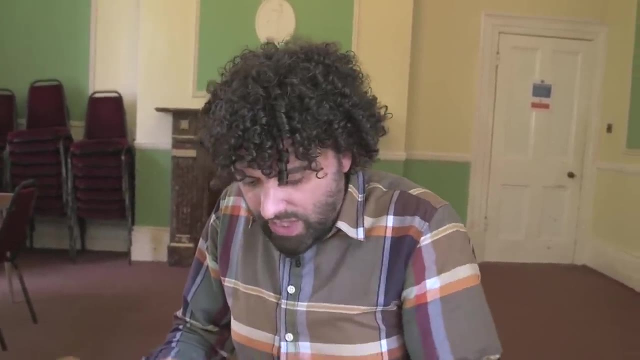 So if we actually think there's a nine right there in the two hundred and fifty-fourth position, So what would that mean? That means that we're actually taking away one with this many zeros. So we've got to imagine there's a one here and then it's got all. 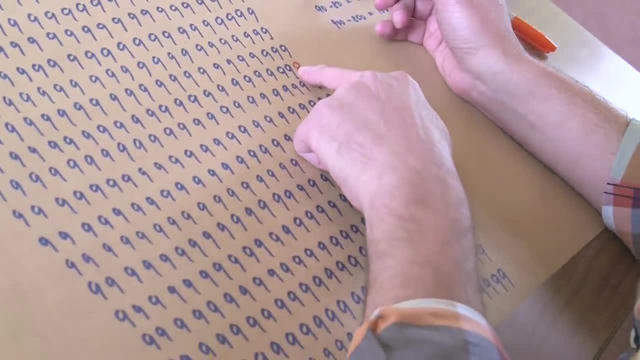 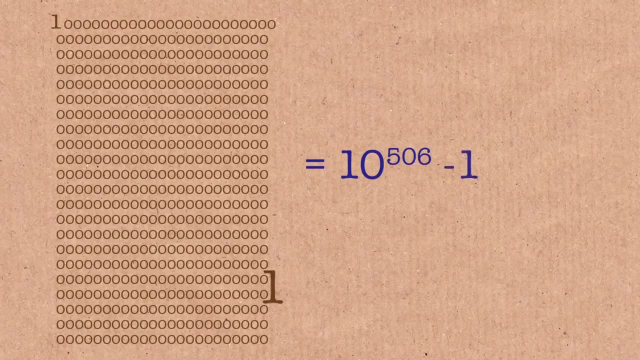 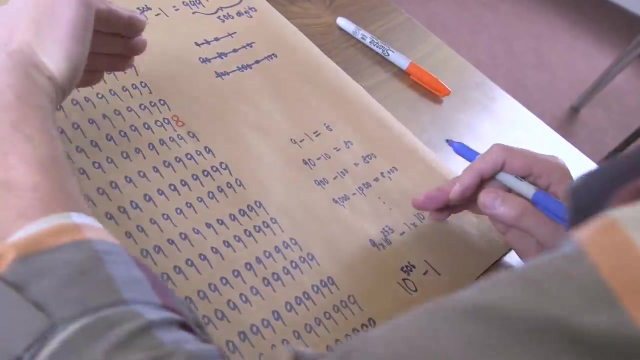 For every nine there's basically a zero, because that's continuing what's going on here. So now what we're doing is we go ten to the five. zero six. take one, gives us this sea of nines, And then we just want to take one with a whole bunch of zeros to kind of get it up to that. 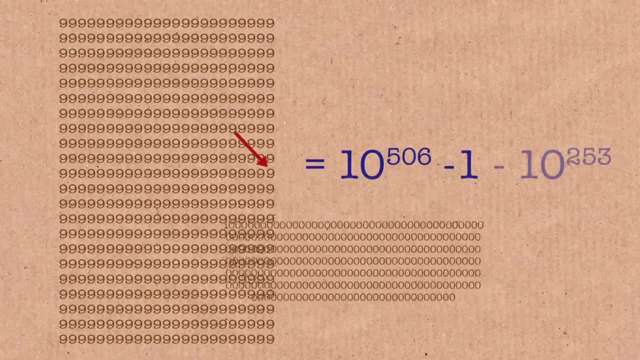 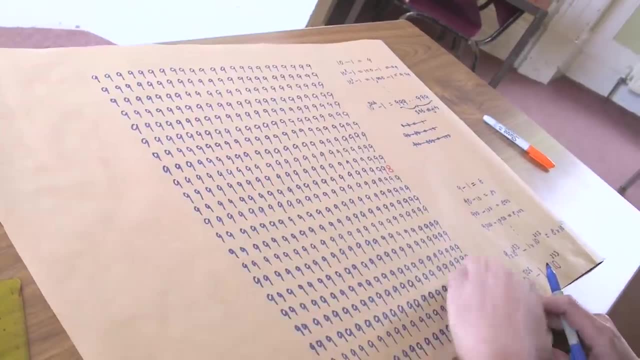 point there. So we're basically taking away ten to the two hundred and fifty-three, So that's what that's equal to. So it's that, take one to give us the nines, take that to take one away from that spot. 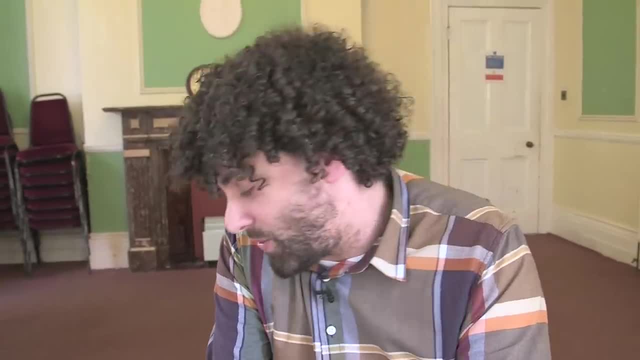 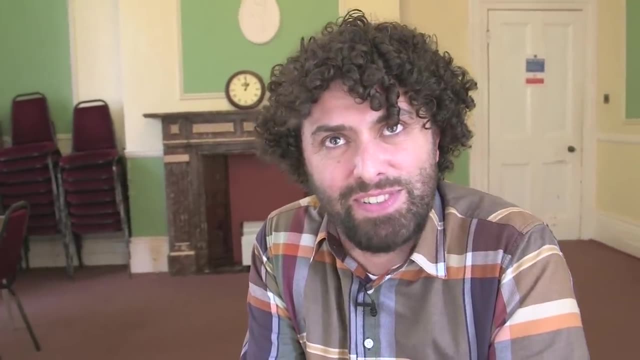 So yeah, So that's the kind of way to actually carry it around and talk to your. This is the way you talk to big numbers, big prime numbers, like this to your friends. You don't go 999999999 and some sort of Ali G refererемentry here. 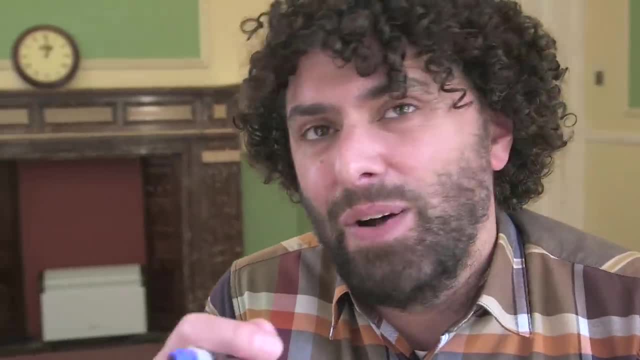 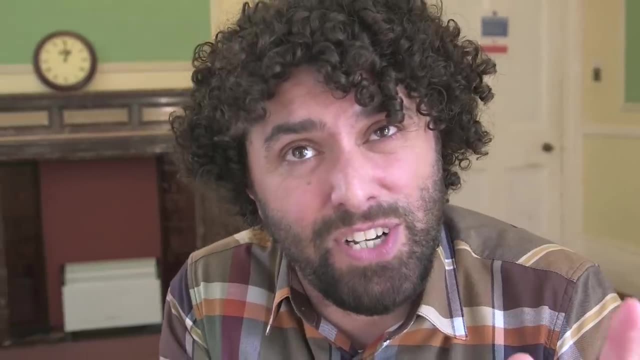 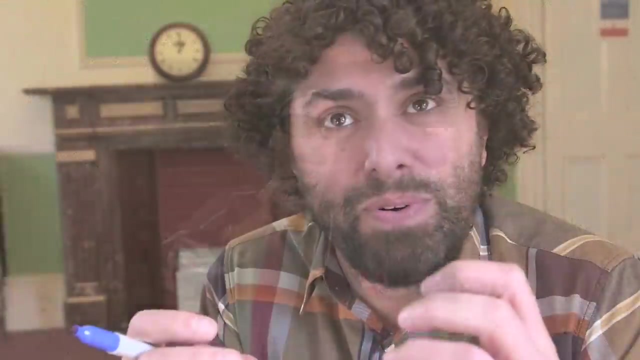 Which is interesting. In actual fact, Ali G does this thing. where he goes, he actually does this and i actually counted the number of times. he said nines and eights, nine, nine, nine, nine, nine and it's unbelievable. he's like one off, one place. 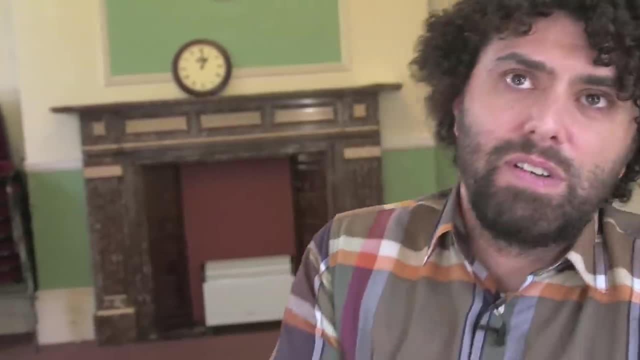 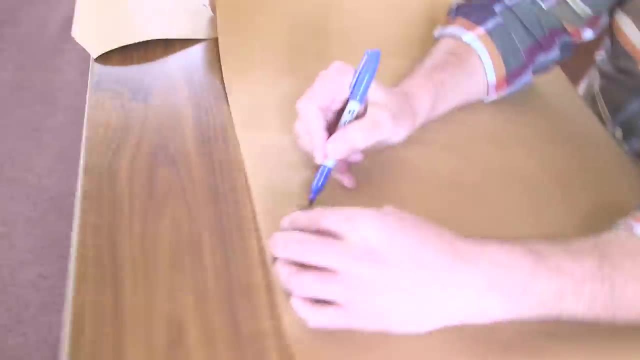 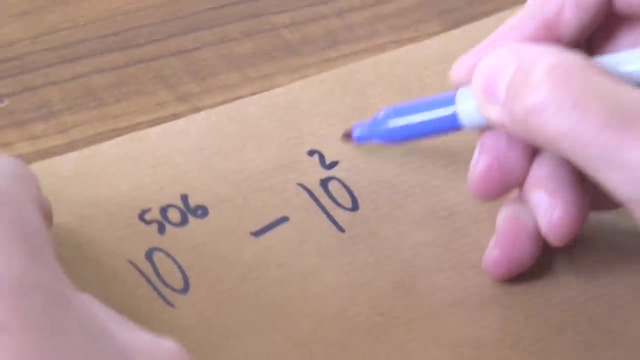 off actually having one of these glitch primes. that would have really made the nerds excited. so now what we have is a way to actually understand this number. so now we have 10 to the 5, 0, 6 take, and I'm just going to order it in terms of: 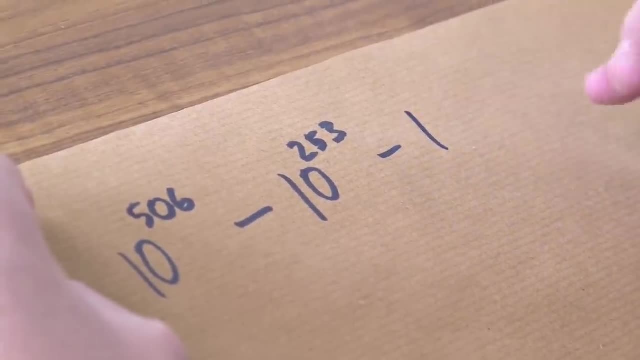 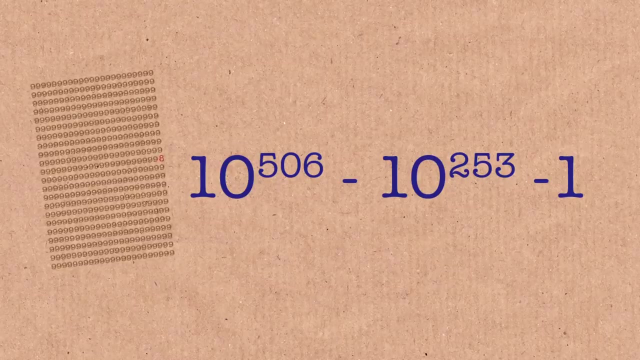 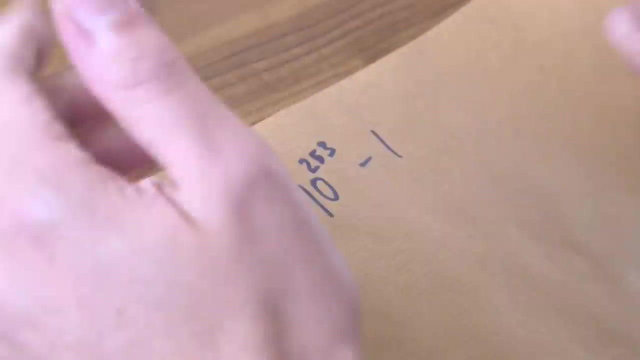 magnitude here. take that, take that basically what you, what you need to notice here. what's going on is the fact that if you double 2, 5, 3, 253, guess what you get- 2, 3 is a 6 to 25, so it's actually that number. so now we can. 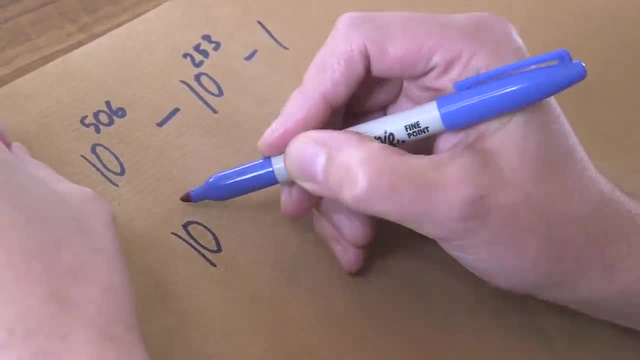 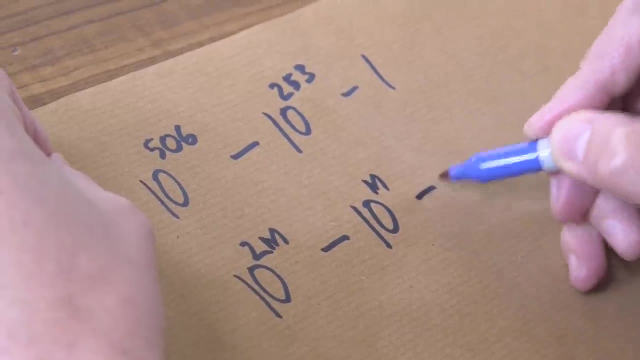 actually find a structure. so I'm going to put in a couple of letters here to denote other things, so I can actually make it even smaller. if you check this out, maybe not, this is in actual fact 4 m. don't you love mathematicians? let's just make it more. 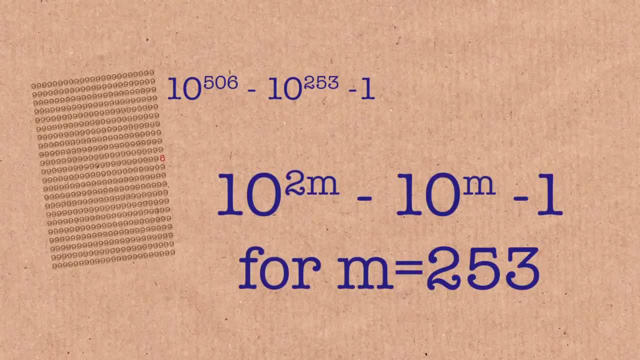 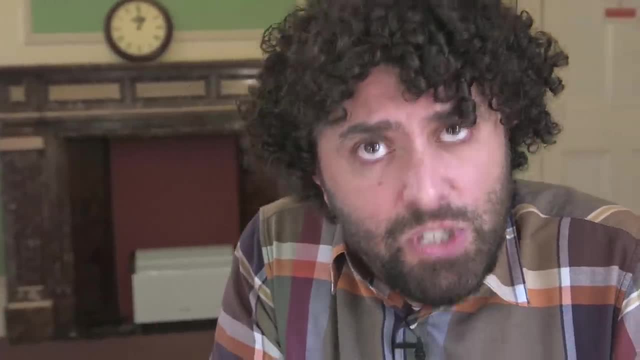 more complicated. so in actual fact, it actually has this shape. so what happened next? I started doing this at 9 pm. I mean I was. I was still doing it at 6 am. I mean I was going down. this is the hole I want to take you down. so now what's? 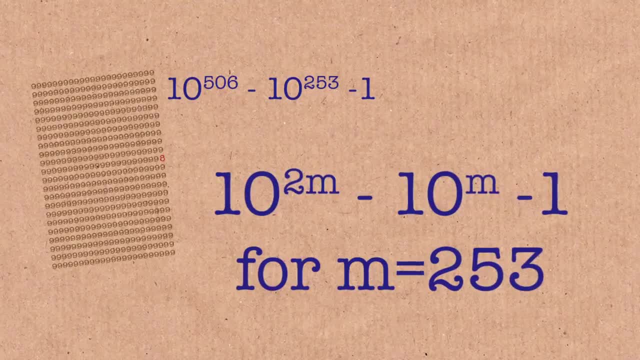 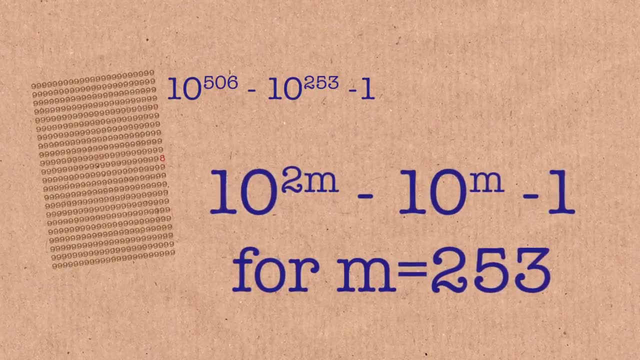 really interesting is that if you, if you learn about how to factorize polynomials, or even you know factorize things, because this is actually 10 m squared, take 10 m, take 1, so you kind of get this taught at school, you know it actually has the 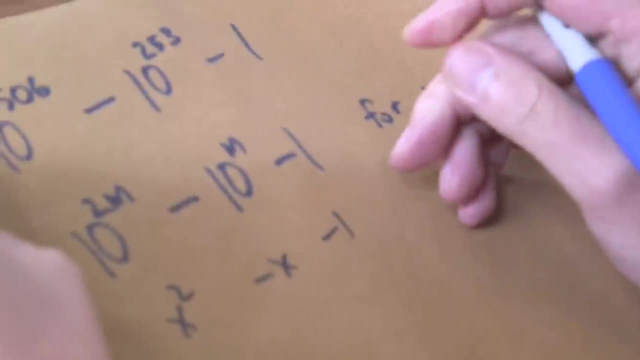 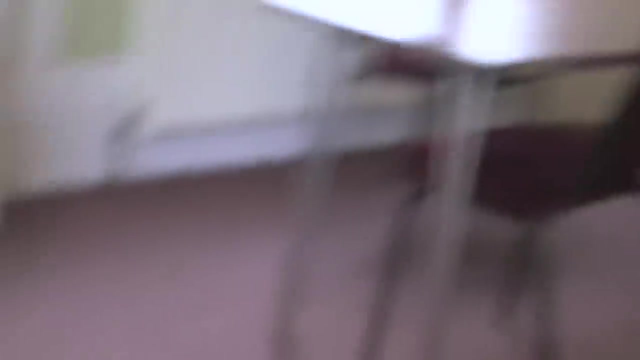 shape of x squared. take x, take 1. so you could actually think, oh, maybe I'm going to be able to work out a way to see when this is a prime or not see. this is what's amazing about these primes. primes don't act that way. 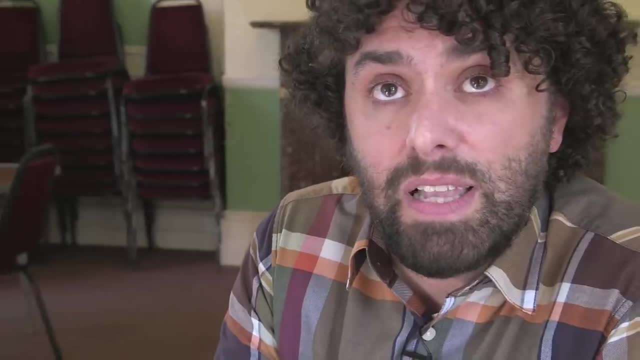 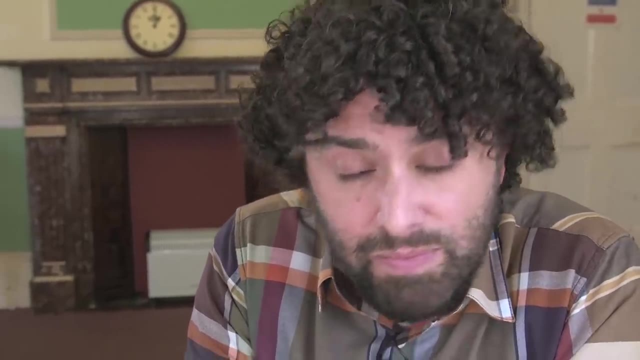 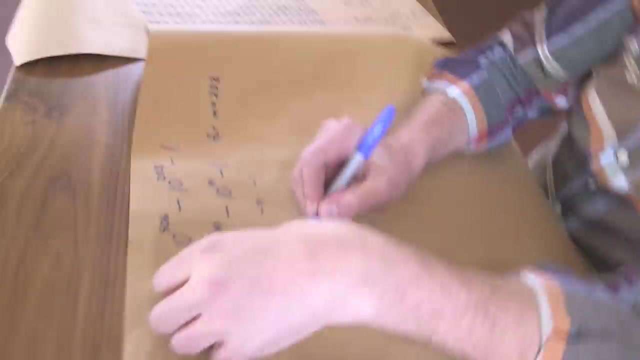 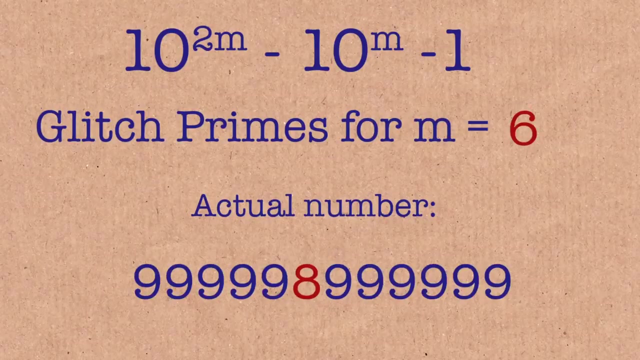 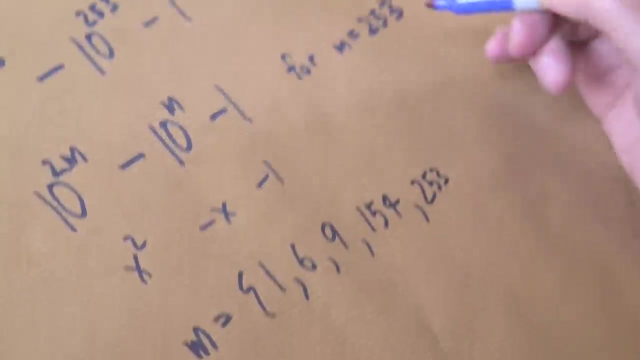 natural fact. I needed to put this number into like a database that would crunch it for me and you wouldn't believe. there's only a small number of M's which will actually give you this particular shaped glitch prime, and they happen to be the values of M, where M is equal to 1, 6, 9, 154, 253. hello, one thousand one. 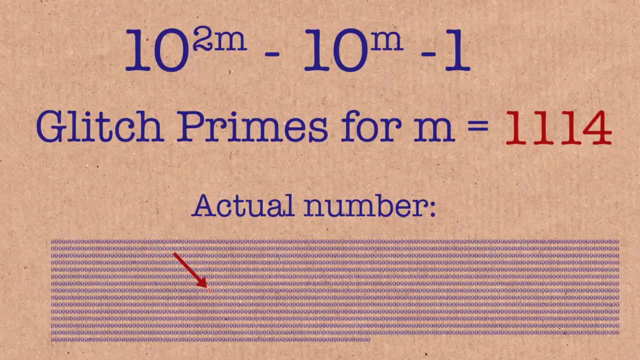 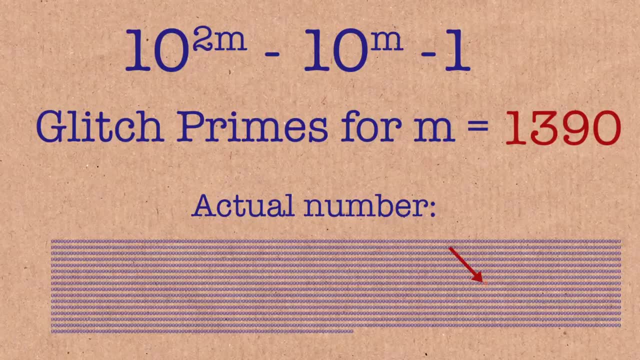 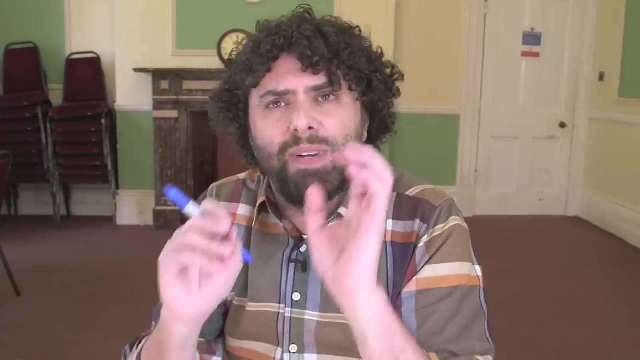 hundred and fourteen and one thousand three hundred and ninety-five, and that's as far as the database went, and I think that's probably as far as we know at this point for this particular. so look at that, think about how big this number is, how many values of M you can have, and it's only for these numbers. 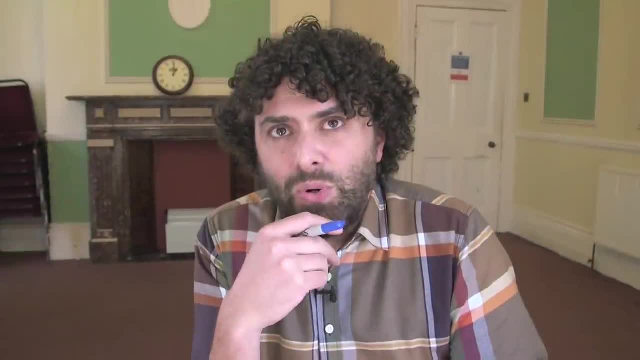 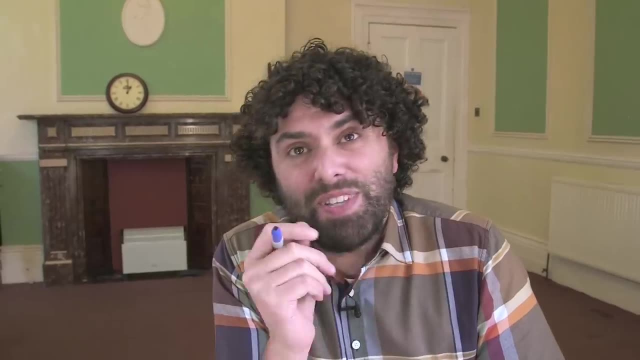 that this will be prime, and that happens to be prime. what's cooler than just a glitch? if so, glitch well, maybe. but maybe also what happens if the glitch was right in the middle of the number. so I actually looked into that as well. so that's a different formula. 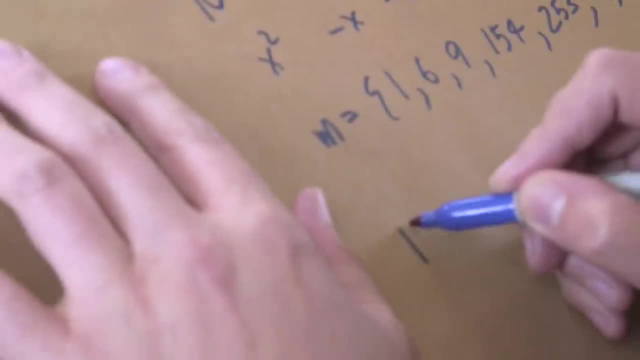 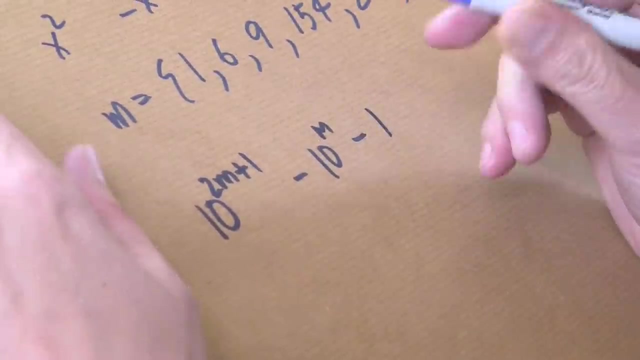 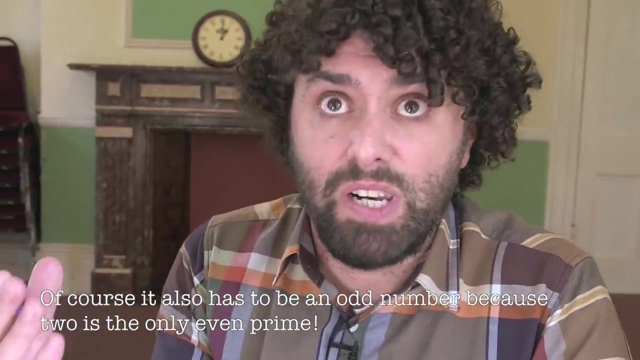 so that formula then is: we're saying it's 10 to the 2m plus 1. take 10 M, take one. it basically has to be an odd number of digits, not an odd number, but in terms of the number of digits it has to be an odd number because it has to have a. 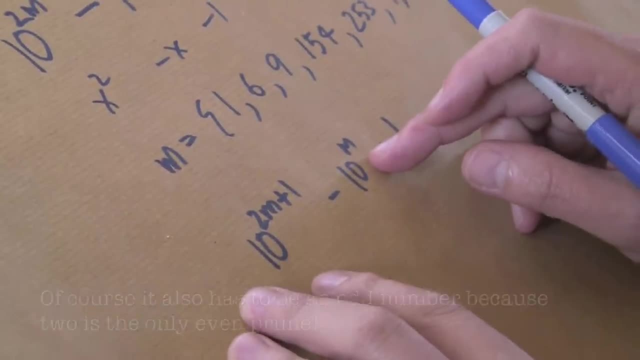 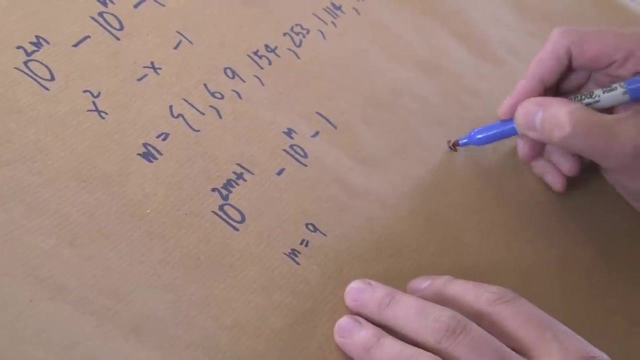 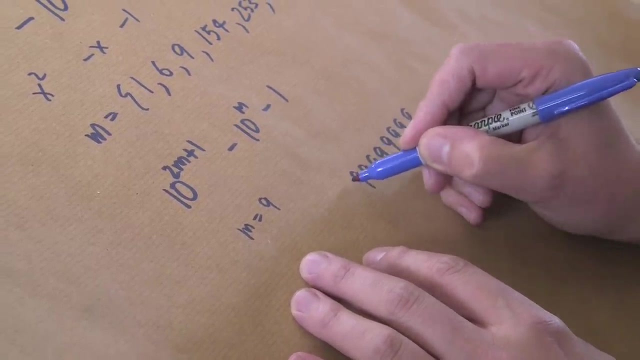 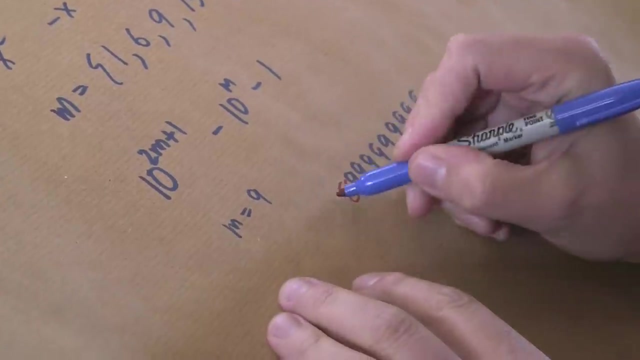 middle. so there are lots of different values for that, but there's actually a really nice value. the first one we can find is actually M equals 9, and so what it looks like is one, two, three, three, four, five, six, seven, eight, nine, eight, and then one, two, three, four, five, six, seven. 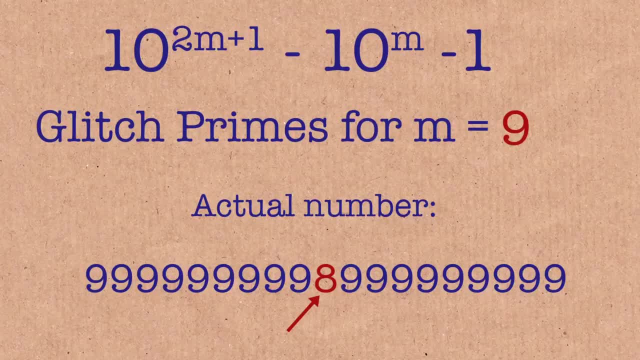 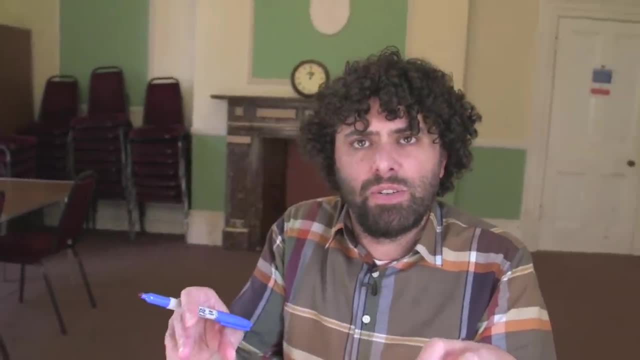 eight, nine. So it's nine, nines, eight, nine, nines. Come on swish. But see, I looked at this and I thought glitch. What are glitches? We think glitches, we think computers, we think binary. 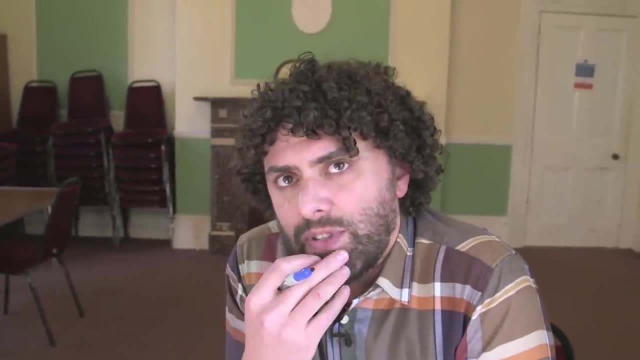 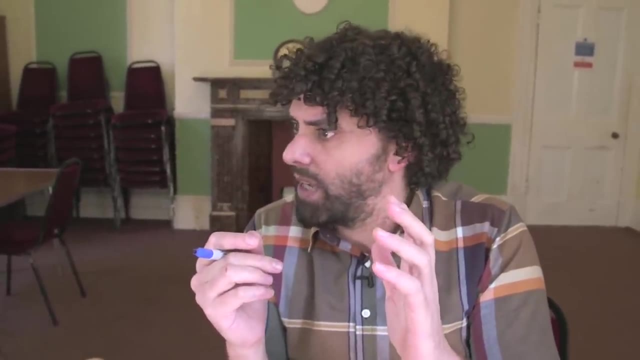 So really, where this took me to was like I'm looking at these glitch primes the wrong way. I should be looking at binary glitch primes, So I want to look at binary numbers. So, in that fact, in that case, I'm looking at, instead of nines, I'm looking at one, one, one, one, one, one one. 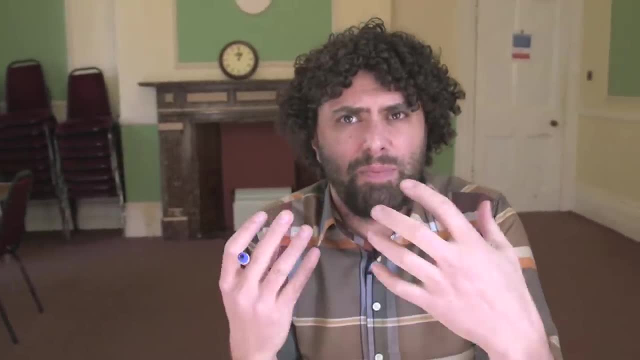 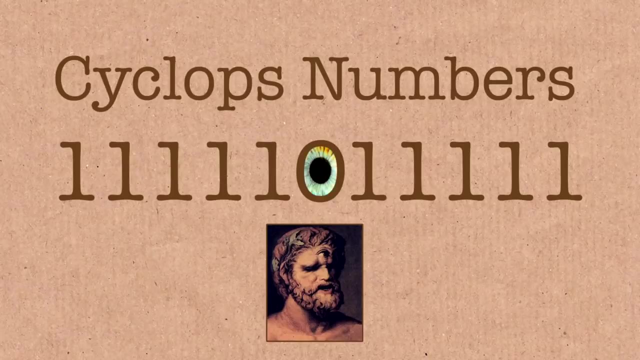 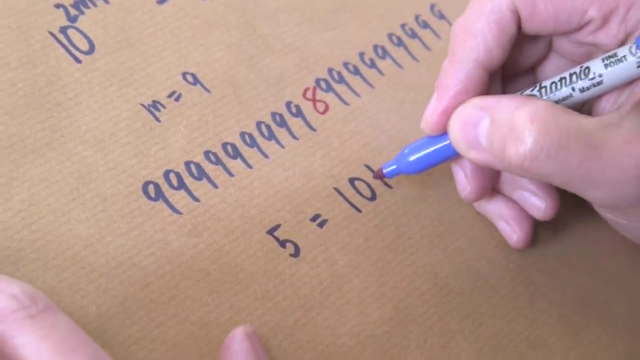 glitch, one, one, one, one, one. And also, let's just think about the coolest thing: a palindrome. And they've actually got a special name: They're called cyclops numbers. So for a, For example, five is one zero one Cyclops because it's got a hole in the middle. But you've 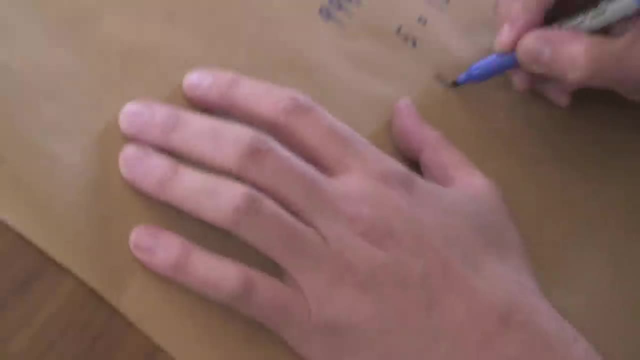 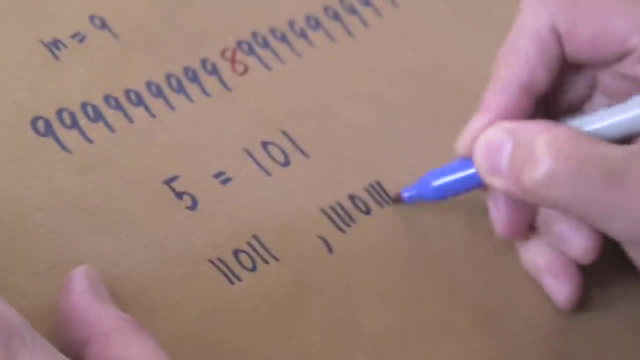 got lots of other cyclops numbers. I mean I don't even have to work it out. You could have like two ones and a zero and two ones, whatever that is. Or you could have three ones and a zero, three ones, Or you could have like four and a zero and four. I mean this is getting you know. 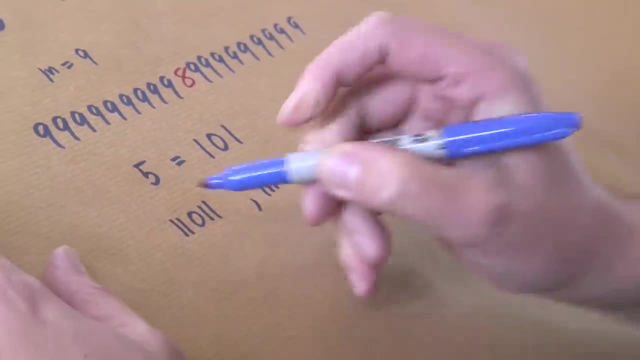 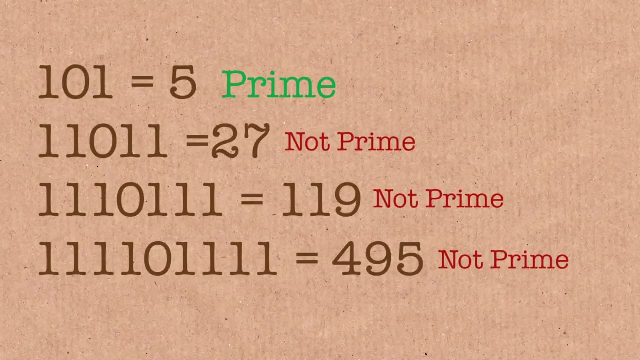 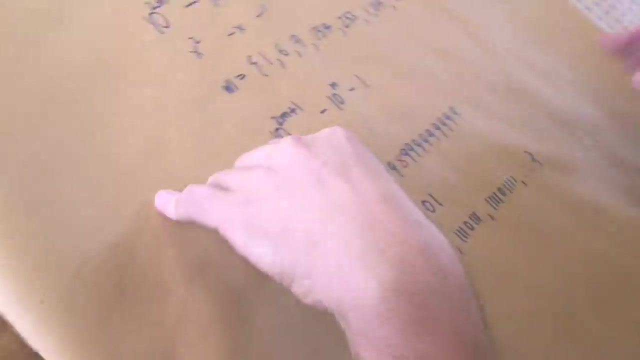 we're really. I mean, this is the sort of stuff you communicate with aliens about. you know what I mean? Well, that was my question. I wanted to know if other ones could be prime. And this is really where my mind was blind, Because I then had to change the structure of this thing. here It's 10. 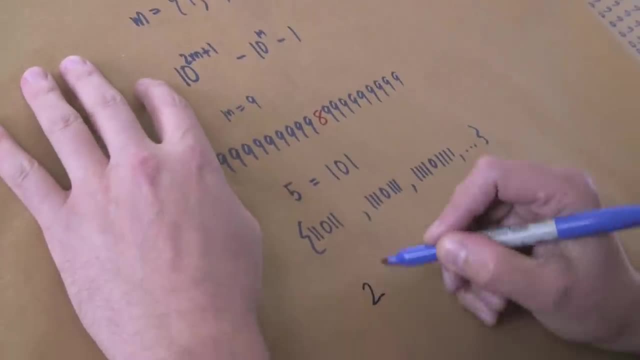 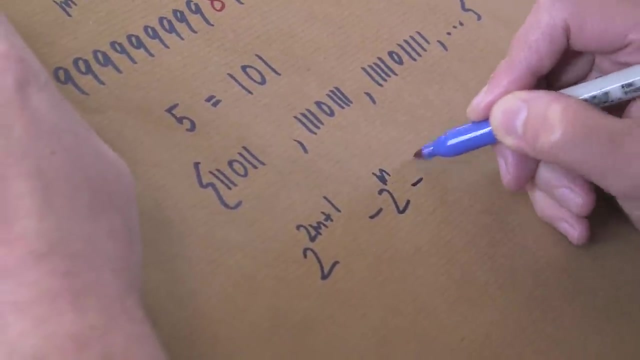 because it's base 10.. But if we actually do it like this, so if, then if it's 2m, because we're basically doing it in binary, so that just means that we need to do it in power two right What? 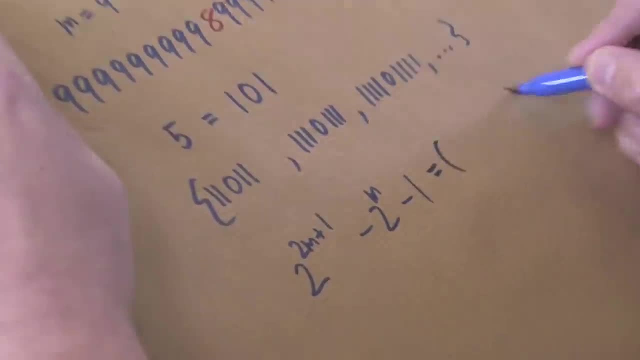 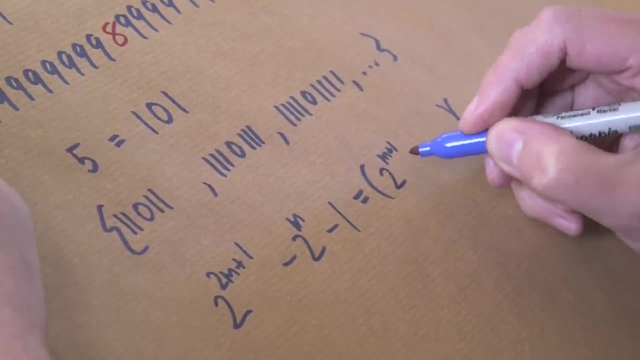 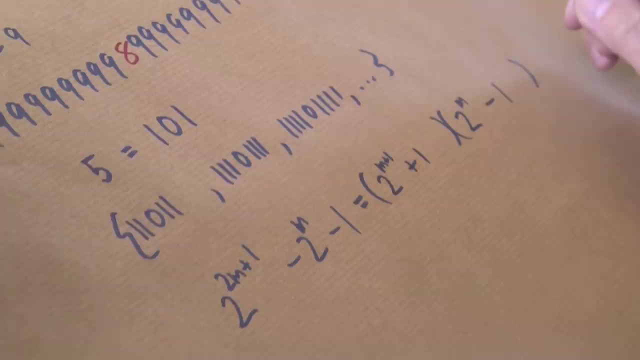 that means is: This is unbelievable. I'm able to actually factorise this into 2m plus 1 plus 1 to 2m, take 1.. So you're always able to do that because it's 2. You can't do that with any other number higher. 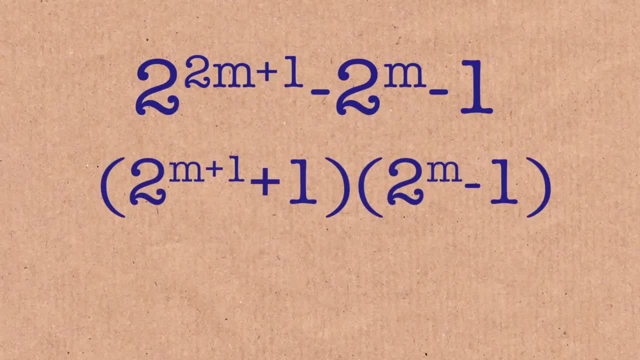 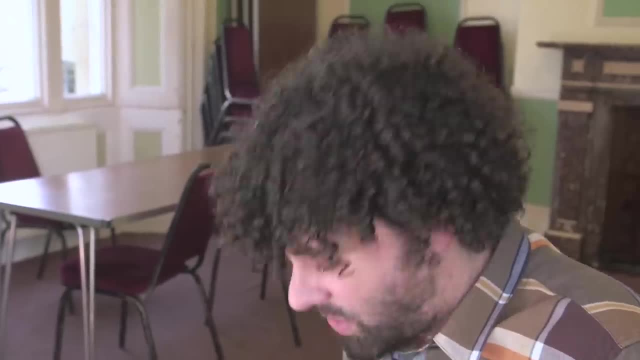 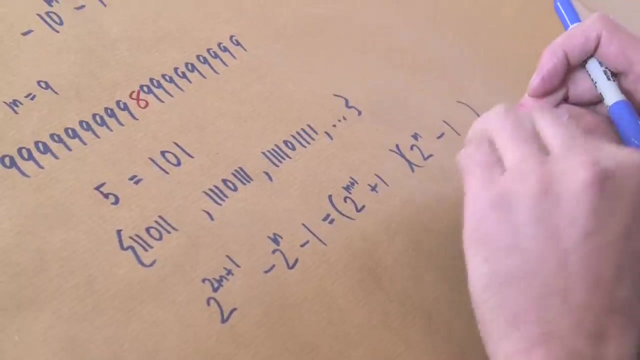 than 2.. And this is a problem, because guess what? Primes, by definition, don't have any factors. They don't have any factors, It's just only divisible by themselves and 1.. So, if you can actually turn this always into this, the only time this is not going to be a prime is when one of 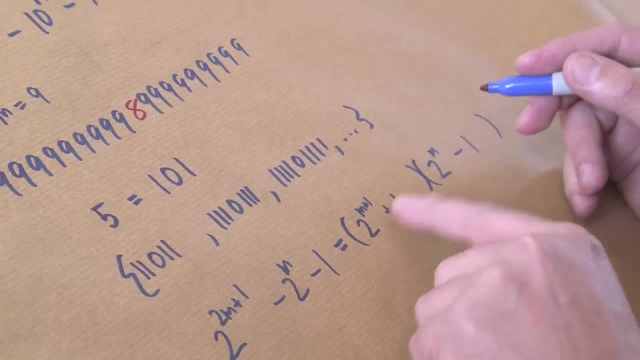 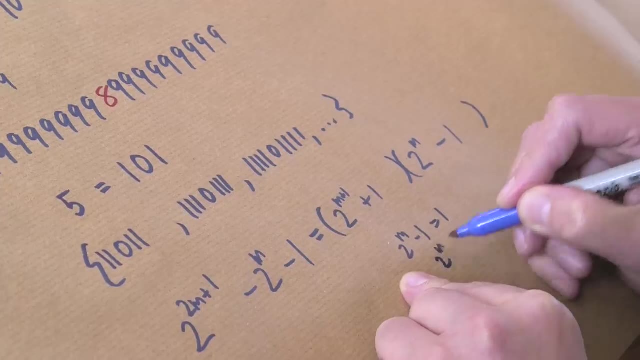 these things is equal to 1.. So this is getting added. It has to be 2m. take 1 equals 1.. So then that means it's 2m equals 2.. And, come on, it's m equals 1.. So that means it's. that means the only. 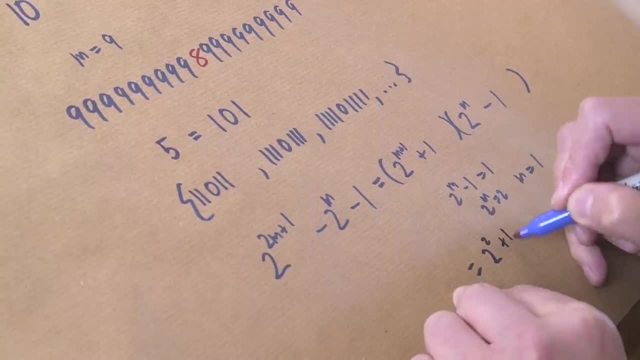 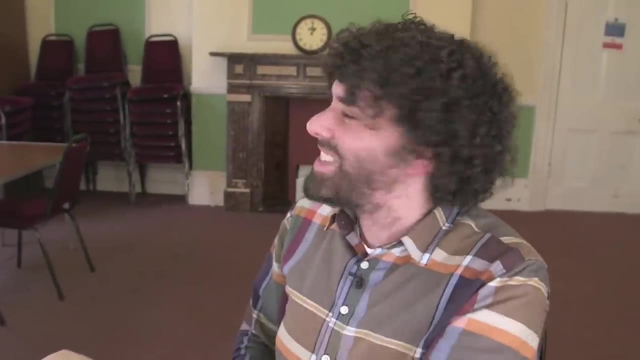 prime we have is 2m, So that means it's 2m equals 2.. So that means it's 2m equals 2.. So that means it's 2m equals 1.. 2 to the power, 2 plus 1, 5.. So where this took me unbelievable, the morning the sun's rising. 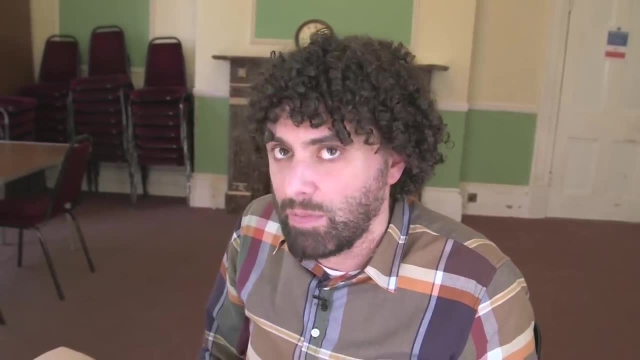 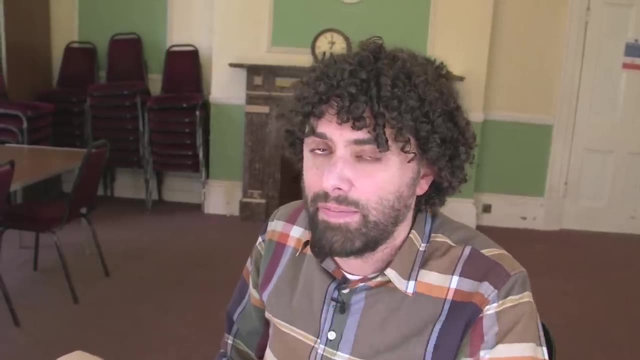 and I realise- maybe I'm the first person to realise- I'm not really, but that's how I feel about maths- that the only glitch prime you can have in binary is 101.. We'd like to thank audiblecom for their support of this Numberphile episode. 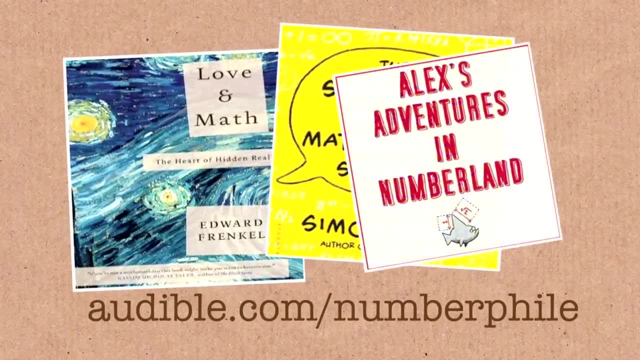 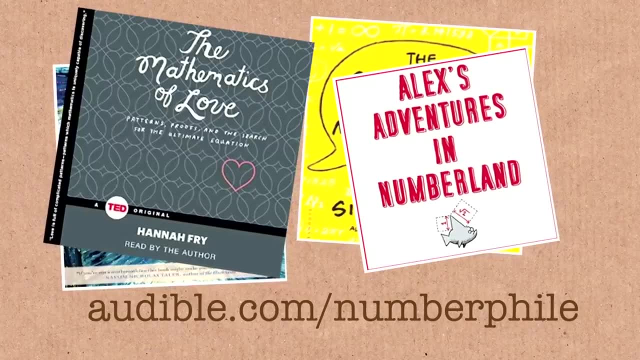 If you want to enjoy a book or other spoken material. Audible has everything you need, Everything you could wish for. They've got over 180,000 titles to choose from, and they're offering a 30-day free trial when you sign up for the service. Now, if you're in the mood for some more, 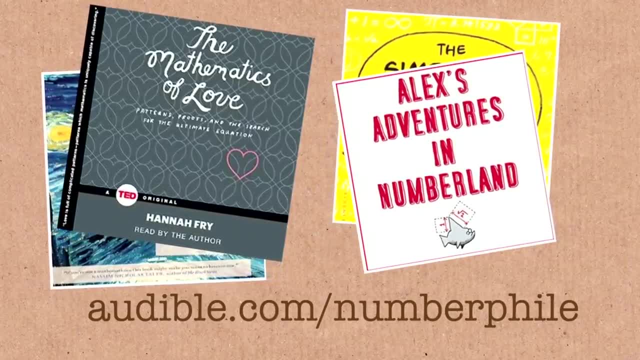 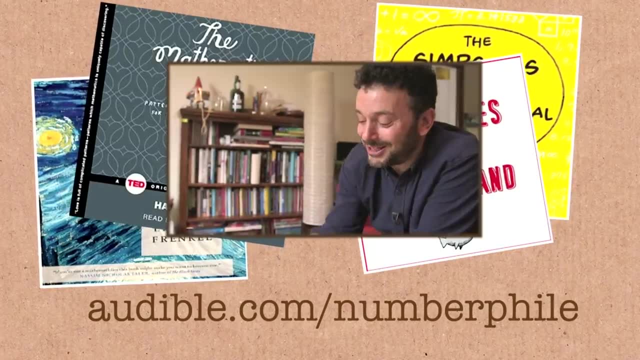 mathematics. I can highly recommend these books on the screen, including Alex's Adventures in Numberland and The Mathematics of Love, both by people who appear in Numberphile videos. Or if all this talk about Cyclops has you excited, why not go old school? 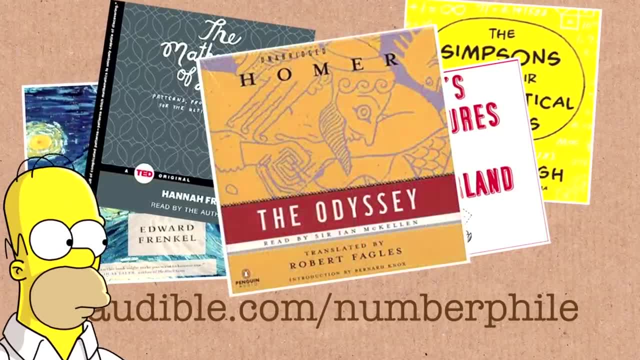 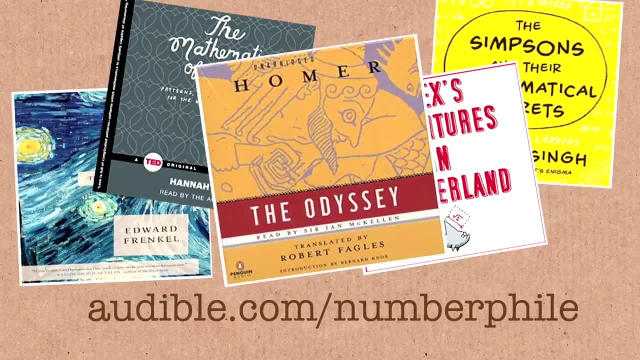 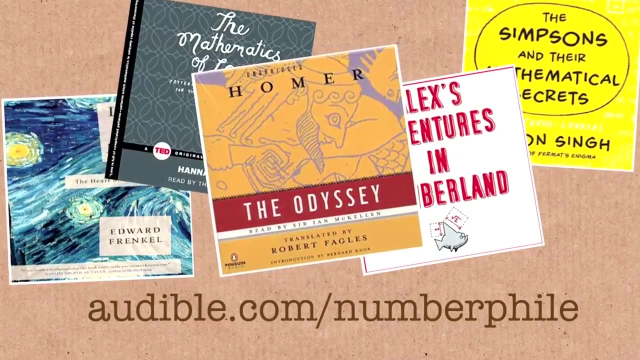 and listen to none other than The Odyssey by Homer. Not that, Homer. If you do check out Audible- and I highly recommend it, I use Audible myself- then use the URL: audiblecom slash Numberphile. That means, if you do take them up on that free trial, the good people there will know you came from here.